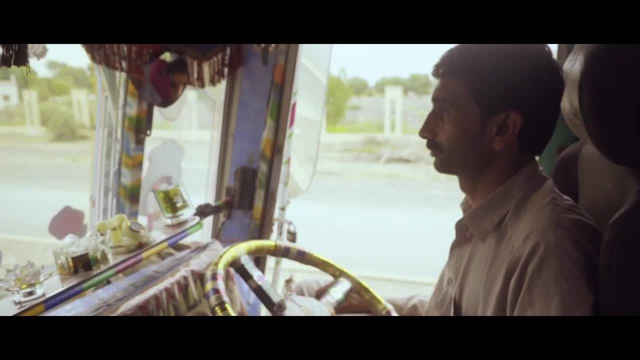 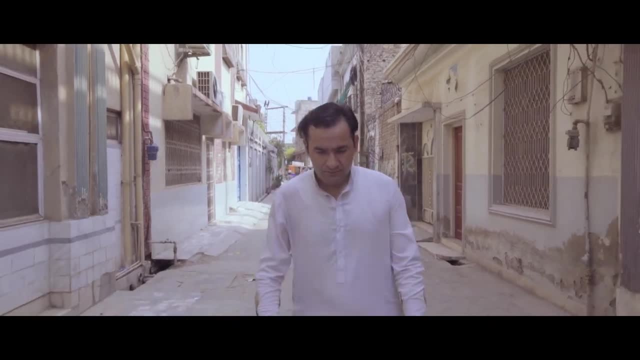 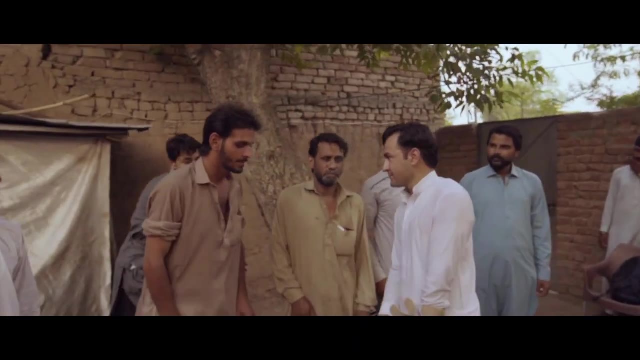 and not accustomed to a woman publicly engaging with them. What gives her this courage? Saddam Hussein is a student of Peshawar University. Out of his own accord, makes visits to engage with marginalized groups of society to enable them to make informed choices for their future. 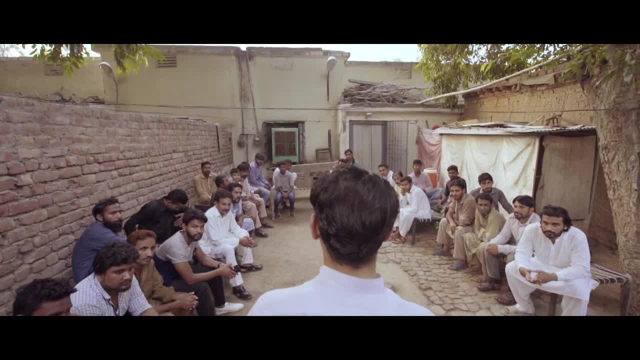 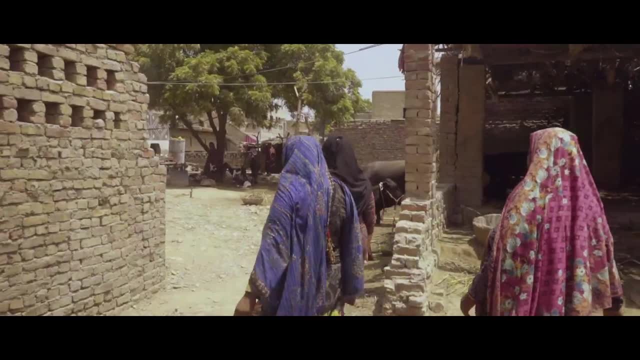 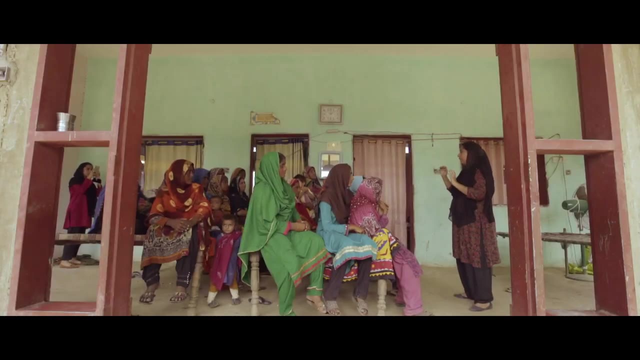 What motivates him to reach out to these groups. Bisma Noor, a student of University of Sindh in Jamshoro, makes time to visit remote locations of interior Sindh to hold community awareness sessions on the significance of women's political participation. 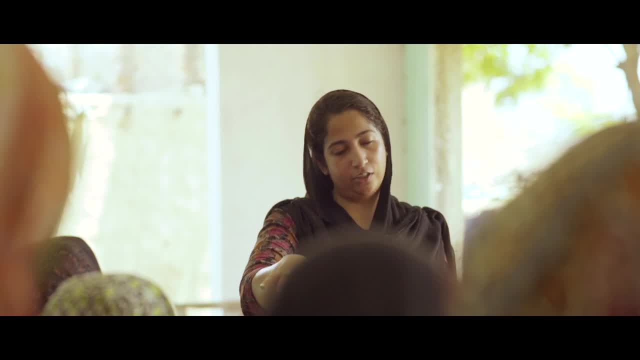 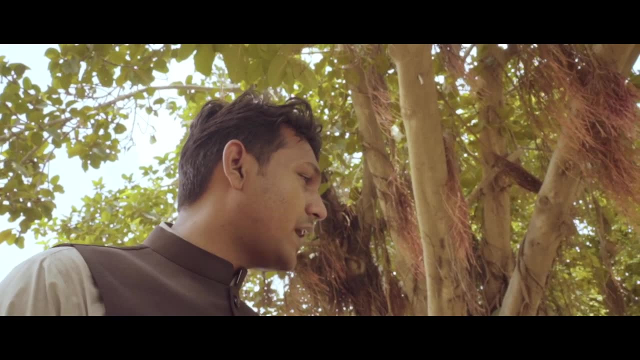 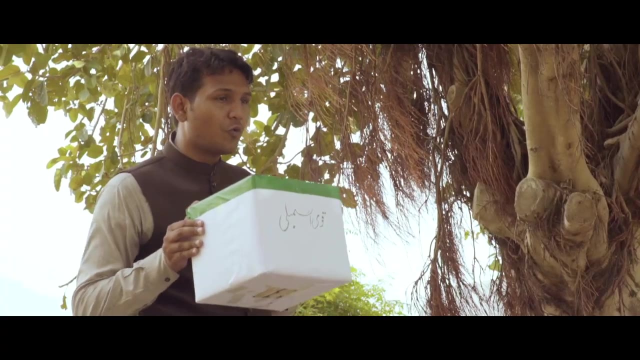 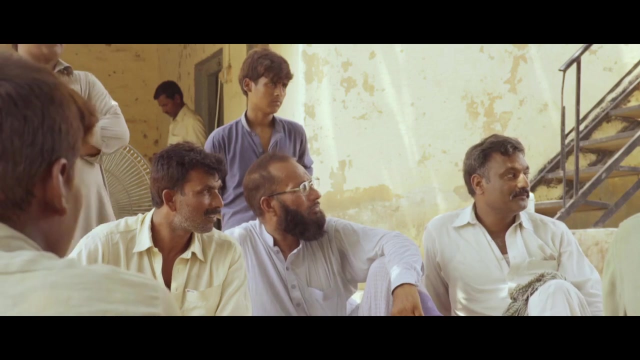 What pushes her to travel to these far-off villages. Imran Shahzaib understands that a democratic society derives its strength from the electoral process And, in order to truly strengthen it, he has made it a mission to educate members of his community about Pakistan's electoral processes and their rights under a democracy. 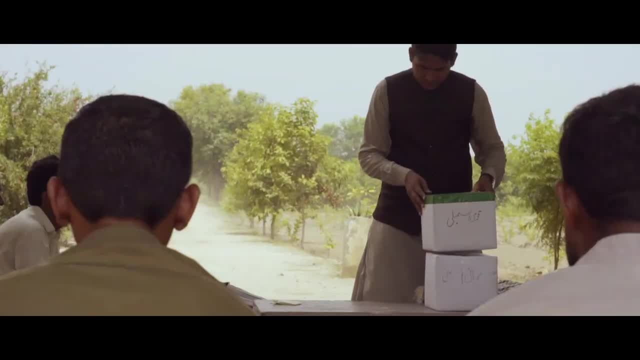 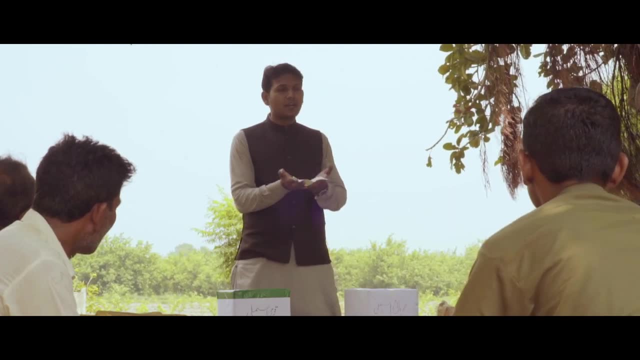 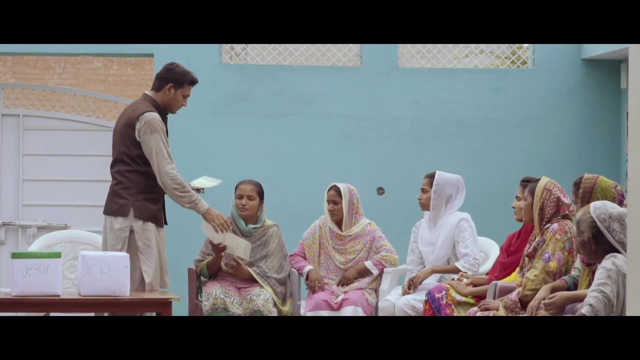 In Multan, Imran visited a rural village and held a mock polling exercise with local farmers to train them on the polling process. He informed them on how to correctly fold and stamp the ballot papers for the candidate of their choice, while also introducing them to the importance of women's participation. 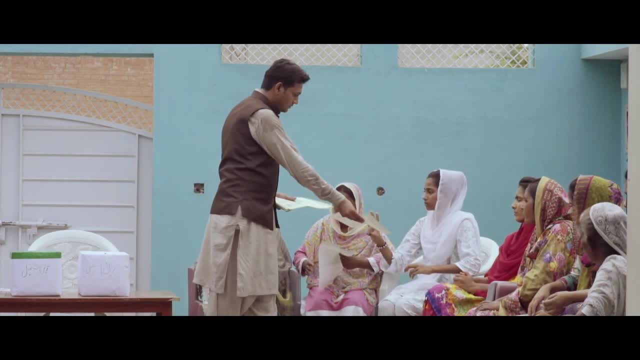 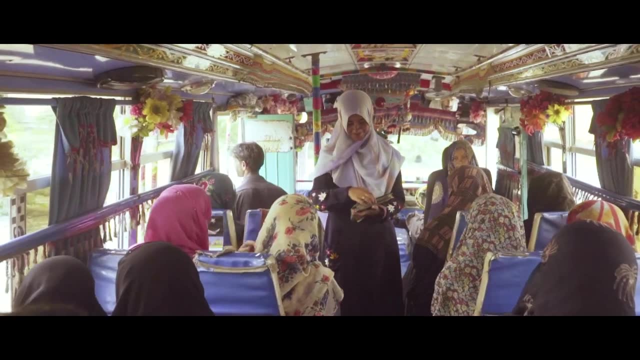 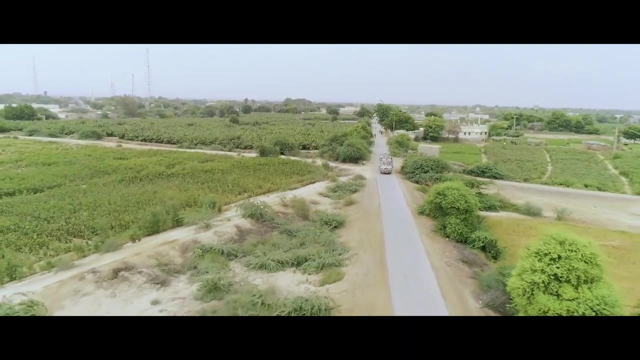 and the need for women to obtain their national identity cards for their ability to vote. Javeria symbolizes women's empowerment in a conservative society, Initiating a very bold and innovative approach. standing in a local transport bus in Las Bela, Javeria delivered an awareness session to the passengers on active citizen engagement. 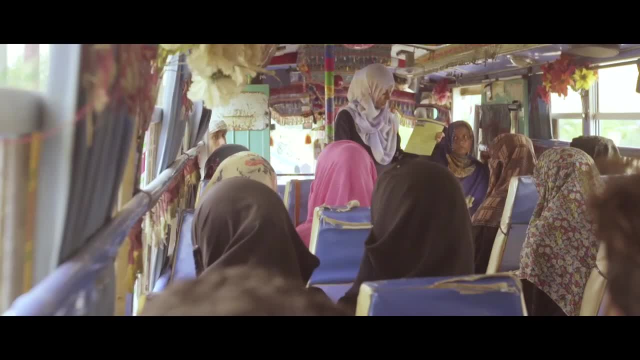 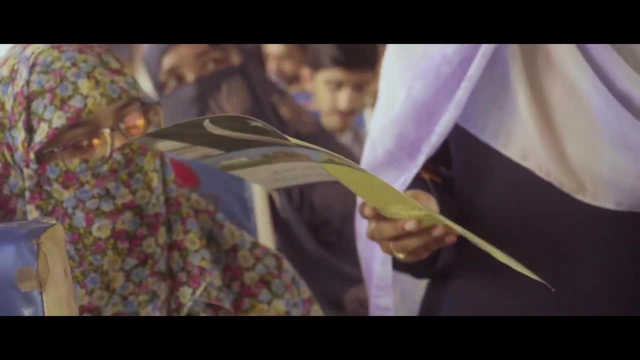 and the correlation and importance of voting in a democracy, including what the government is and how it works at the federal, provincial and local levels. Javeria takes it as her national duty and feels satisfaction over informing people on what they did not know before. 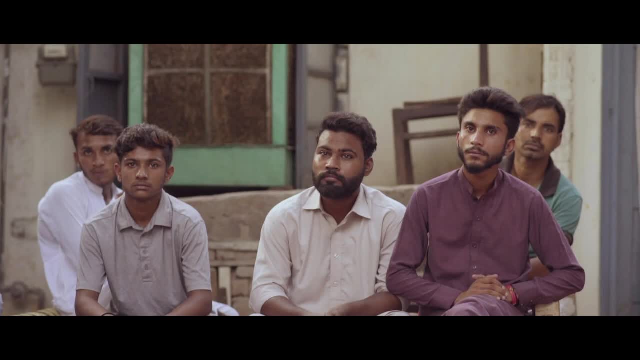 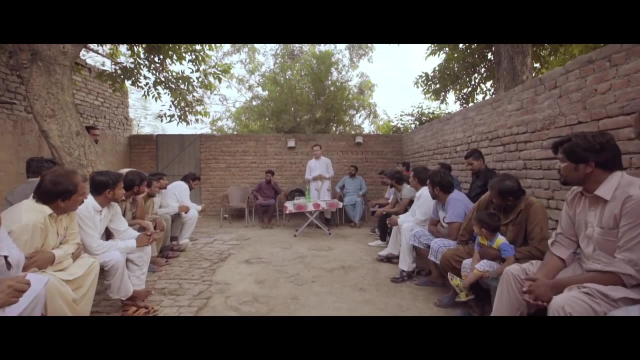 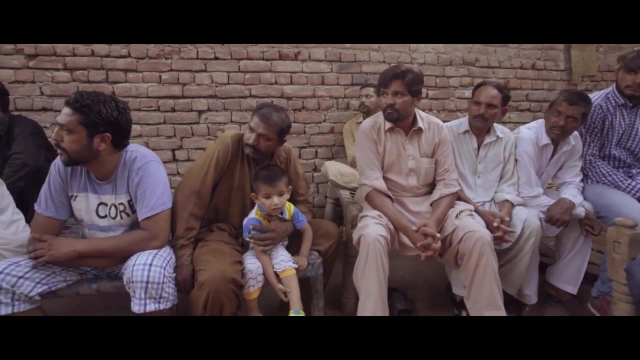 Saddam Hussein knows that every single vote can make a difference. He has made it his mission to promote an inclusive democratic culture, not only for the people he is reaching but for society and the country at large. Saddam promotes that it is in the interest of the country that minorities actively participate. 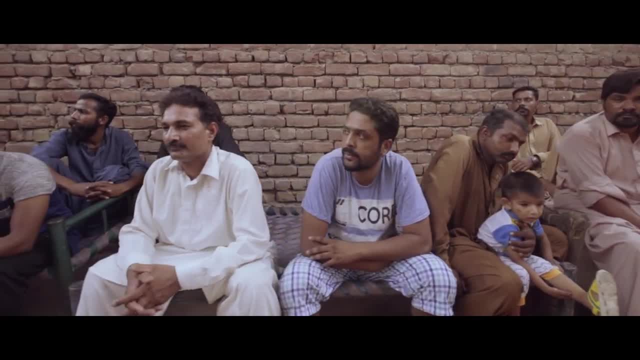 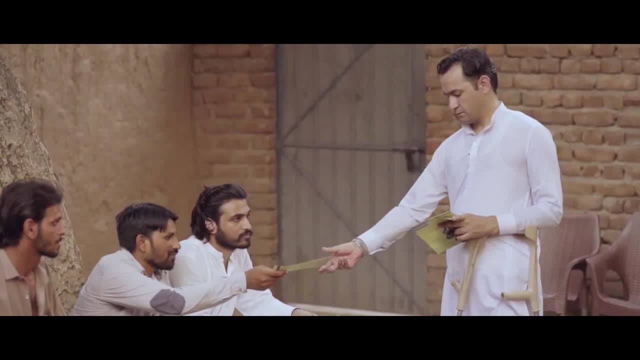 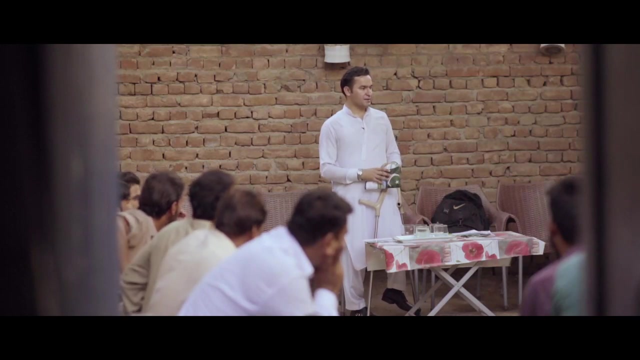 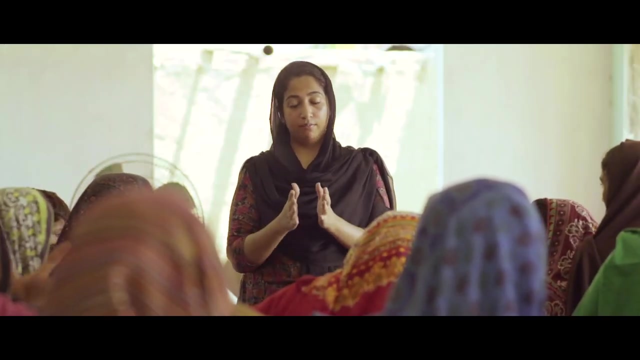 in Pakistan's government structures. In this awareness session and anticipation of local government elections, Saddam engaged members of the local Christian community of Peshawar to emphasize the importance of the local government system in strengthening democracy at the grassroots level. And likewise Bisma Noor understands that women's political and electoral participation. 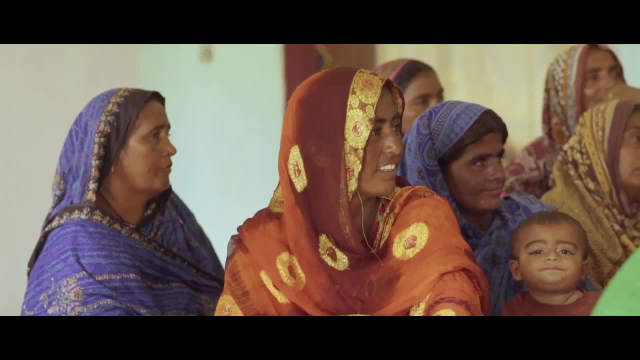 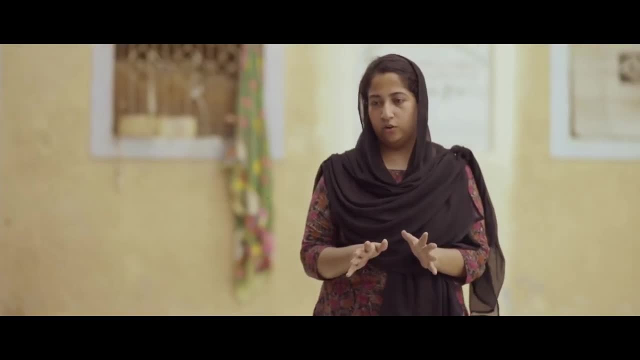 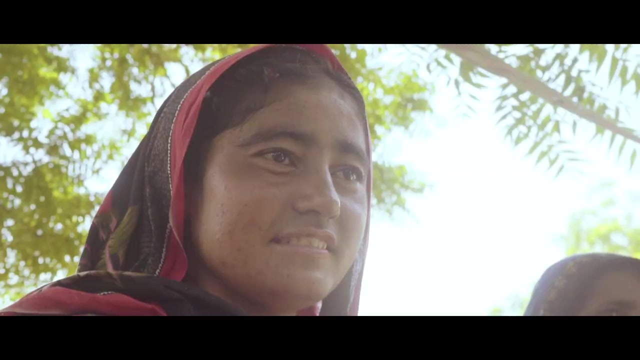 is essential to promoting gender equality in the electoral process. Bisma spreads awareness among men and women of rural villages on obtaining their national identity cards and guides them through the process. She succeeded in getting many young women to obtain their national identity cards in remote villages of Sindh. 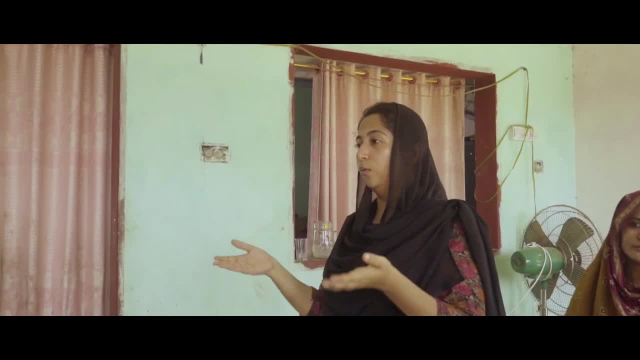 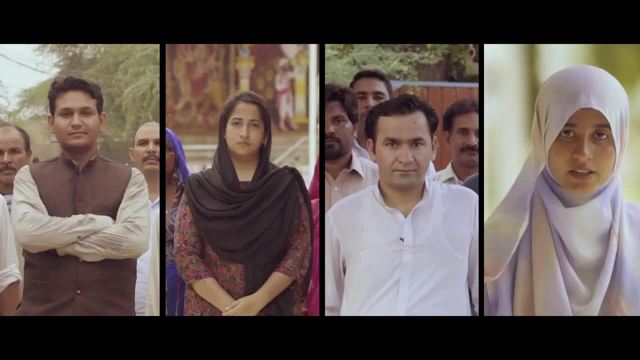 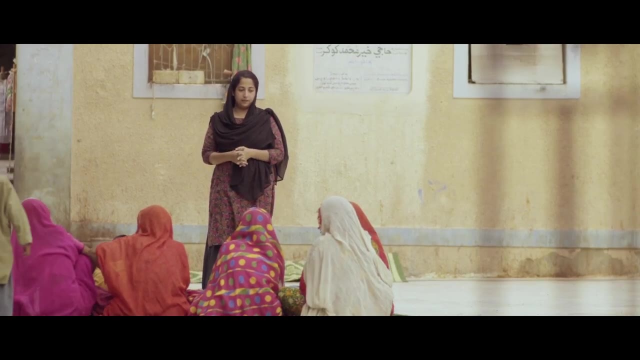 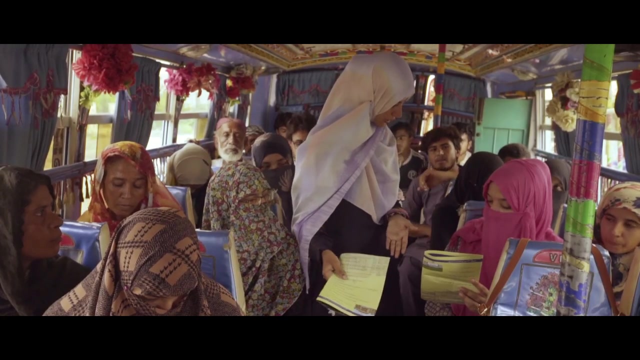 By doing so, Bisma is complementing the Election Commission of Pakistan's Women's National Identity Card and Voter Registration Campaign. These are United Nations Civic Education Youth Volunteers. These individuals represent a small portion of the United Nations Civic Education Youth Volunteers working across Pakistan to promote civic literacy and women's engagement. 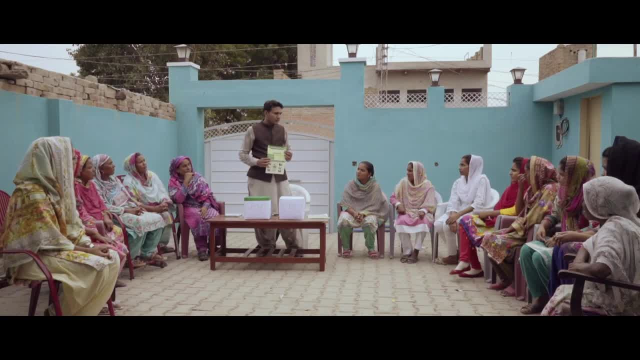 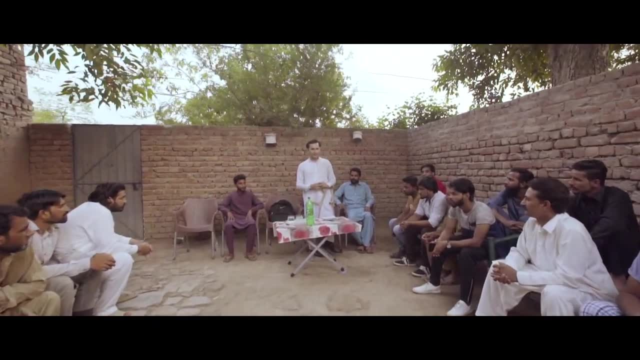 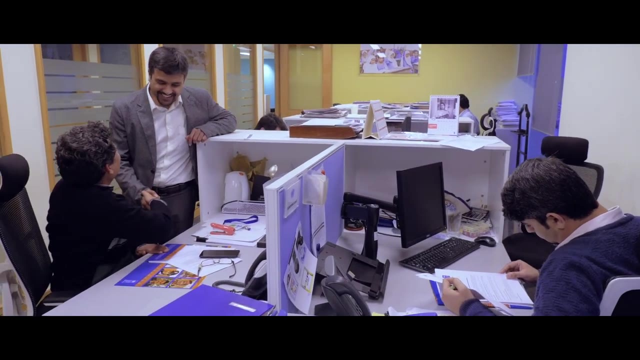 They are not just role models for their communities. Each one of them represents the strongest element of collective action that happens to be the power of one: The United Nations Civic Education Youth Volunteers. My name is Arthur Iqbal. I was one of the first United Nations Civic Education Volunteers. 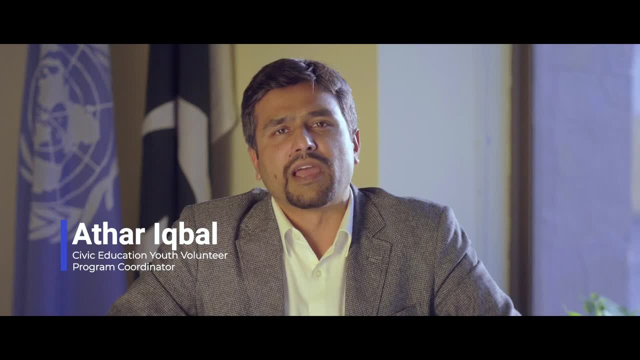 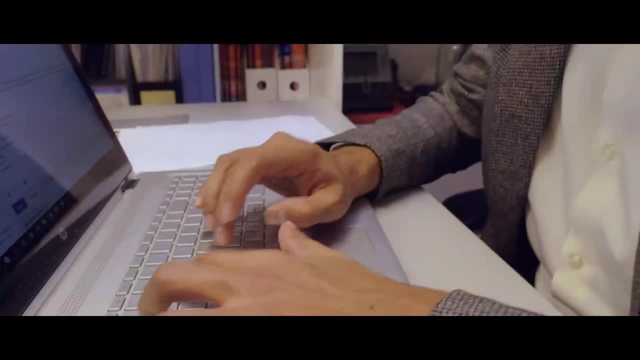 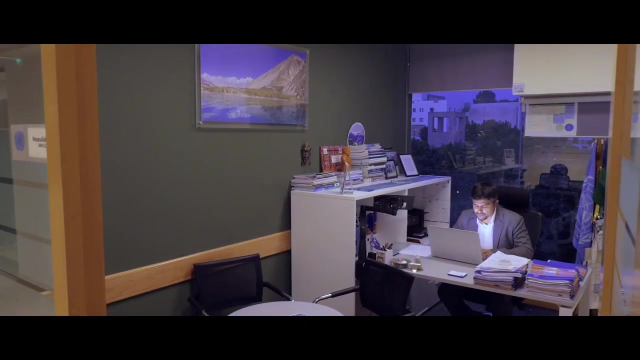 I am proud to now work with the United Nations Development Program and United Nations Volunteers in supporting these and many other volunteers with this important initiative With one of the largest youth populations in the world. this program was created to engage Pakistan's youth in promoting civic literacy. 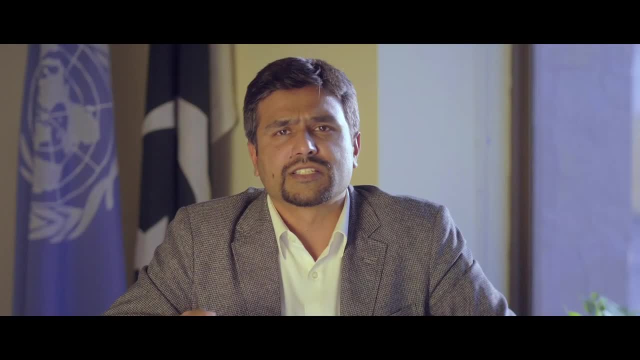 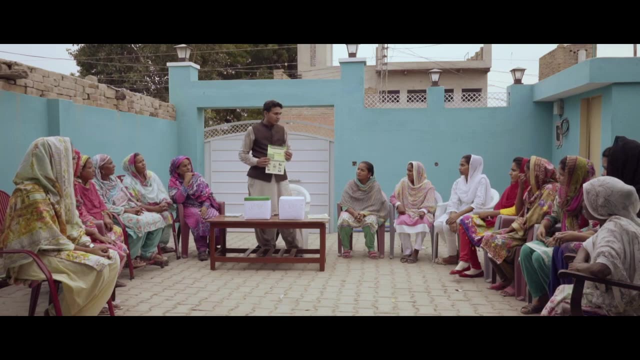 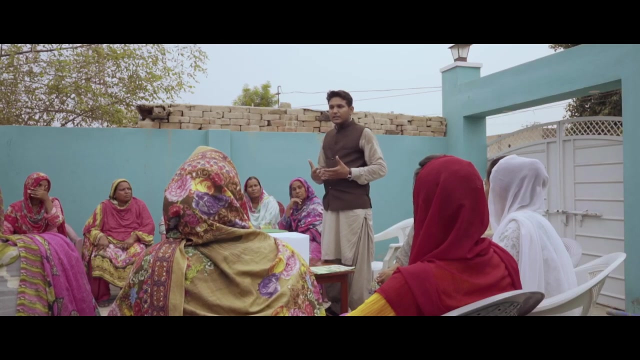 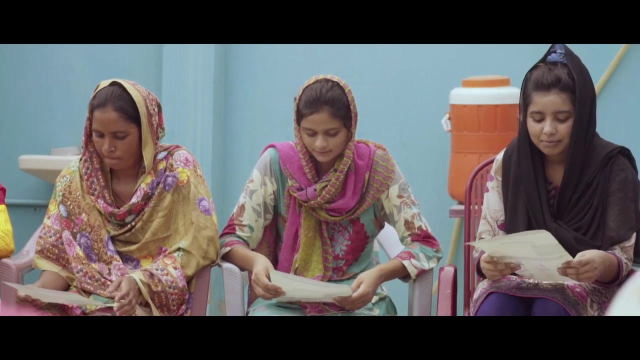 and greater inclusion in the democratic processes, in addition to promoting volunteerism Through brief civic and voter information sessions targeting women, youth, minorities and rural communities. these volunteers represent the power that one individual can make in people's lives. To inspire a woman to obtain her National Identity Card and register to vote,